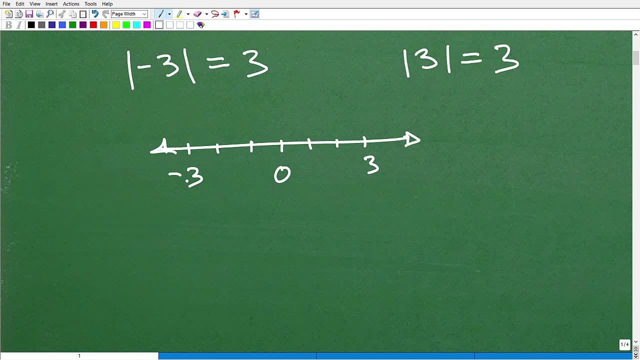 the definition of absolute value is a distance a number is from zero. Okay, the distance a number is from zero. So when I'm saying find the absolute value of negative three, I'm really saying, hey, how far is negative three from zero? Okay. or if I'm saying absolute value of positive three is how far is three from zero? Now, what we're measuring here is distance. Okay, distance, All right. when I'm because I'm asking how far a number is from zero, 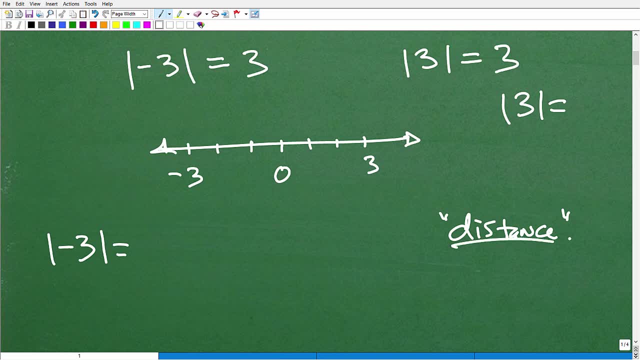 is from zero Distance, like displacement for those who are out there who are like physics, studying physics and whatnot. distance is a always measured in positive values. Okay, Direction, of course you can have positive, negative directions, etc. But what I want you to understand here, for purposes of absolute value, is that we measure distance in a positive way. So it's like, hey, how far is zero from negative three? Well, we take out our tape measure And if I had to, 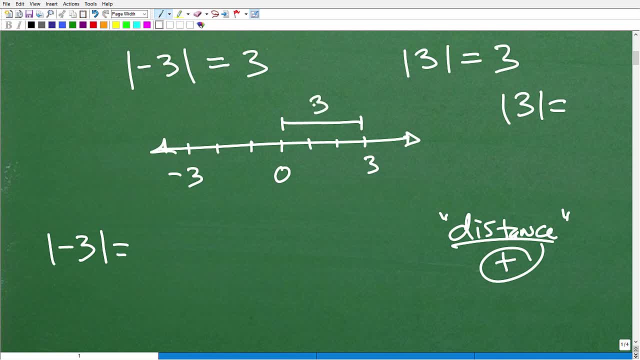 walk this out: one, two, three, hey, it's three units away from zero. okay, makes sense. well, how far is negative three? uh, from zero. well, it's, uh, you know, let's do the same thing. it's, you know, from zero to negative three. oh, it's three units away, but it's in this direction, but nevertheless, it's still. 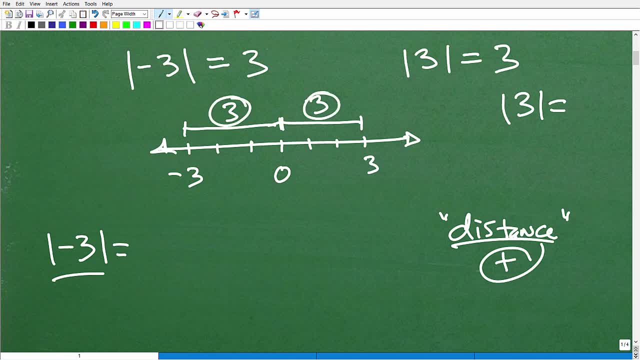 three units away. okay, so that's really understanding what absolute value is. okay. absolute value is indicating or asking how far is a number from zero. this is very important, okay, all right. so now, with that being said, and hopefully that clarified some things, uh, here let's do a little. 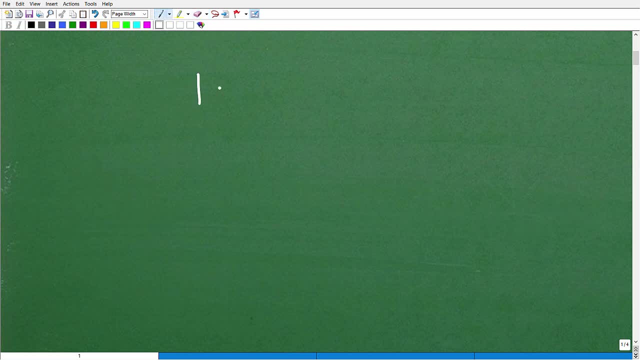 pop quiz. all right. so let's say i want you to solve this equation. okay, all right, absolute value of x is equal to three. hmm, let's see here. the absolute value of some number is is equal to three. what is the answer to this question? well, some of you are like: hey, which? 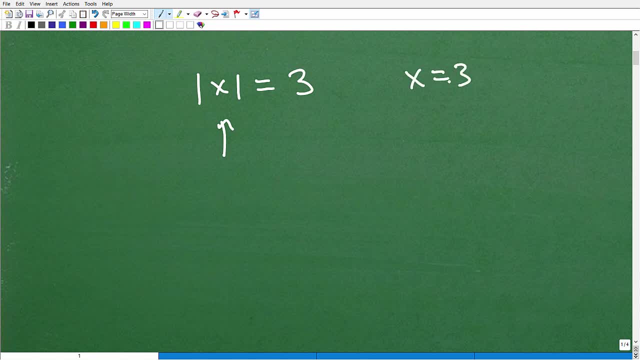 is what we're looking at there. you're like, yeah, you're right, x could be three. okay, you're like, yeah, x could be three, because the absolute value of three is positive three and you would be correct. so x could be three, but x could also be what? x could also be negative three because 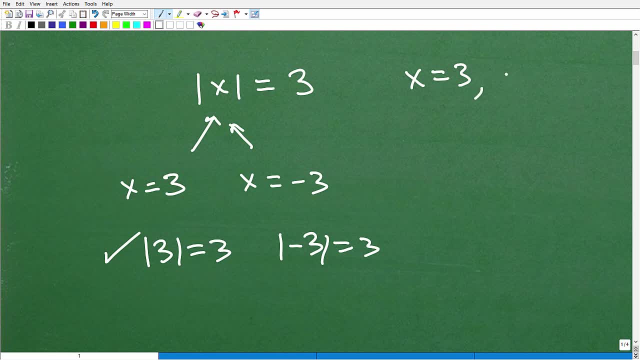 absolute value. negative three is also positive three. so here we have two solutions, and this is the most basic. uh, absolute value equation x is either three or negative three, okay now, now, let's kind of like make this a little more interesting, okay, so first thing i want you to know about 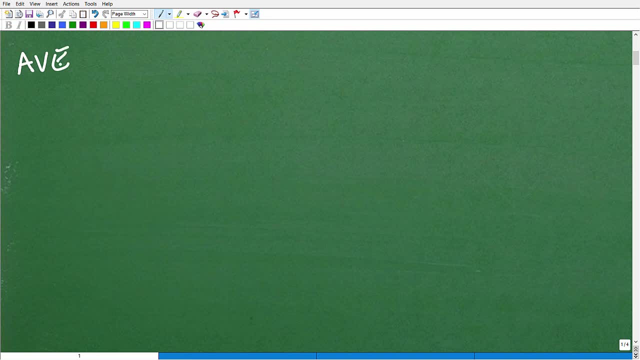 absolute value equations. all right, absolute value equations. uh right, first thing, the number one thing here i want you to know here is that they're always going to have two solutions. okay, just like we just did here. right? so the absolute value of x is equal to three. 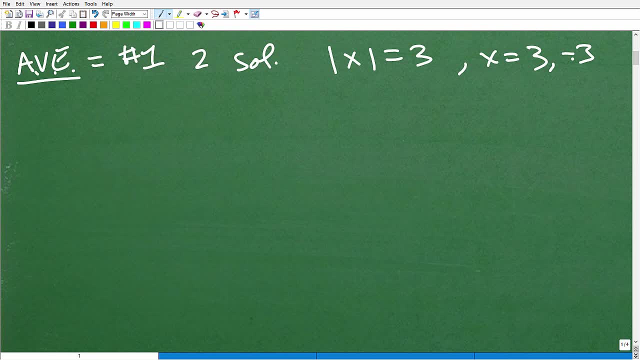 x can either be three or negative three. okay, so the first thing about absolute value equations: always two solutions. right now, what about this? the absolute value of, let's say, 2x plus one is equal to three. how about that? you're like, oh man, this is a little more complicated. well, it is, but let's. 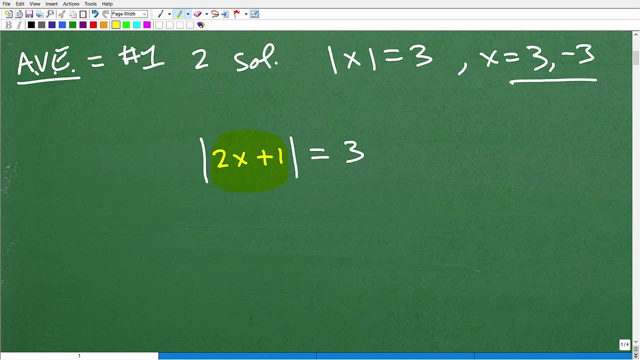 just think about it for a second. all i know is that this guy right here- 2x plus one. i'm like, yeah, 2x plus one is equal to three. and i'm like, yeah, 2x plus one is equal to three. and i'm like, yeah, 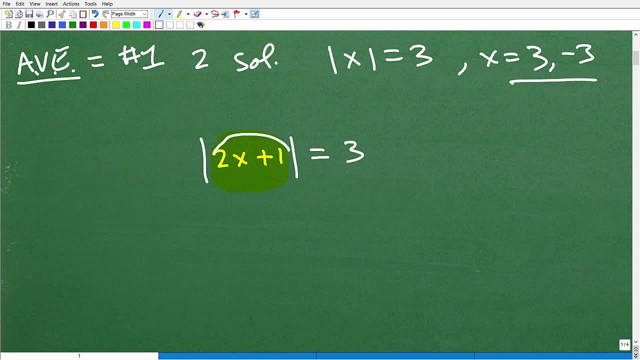 i know you're. you're really in disguise. you're just trying to be a three okay, or negative three. that's what 2x plus one is. it's either three or negative three. of course it's undercover here. it's 2x plus one. it's kind of floating around and be like yeah, yeah, i don't want anybody to 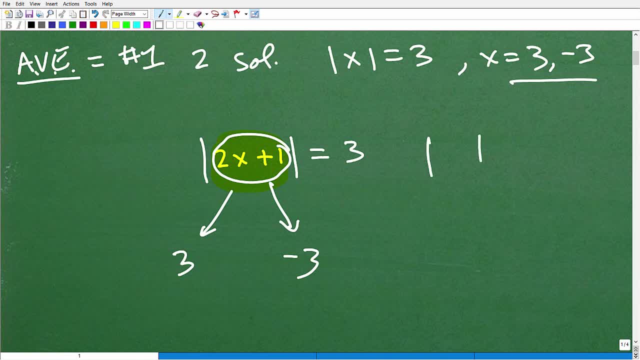 know that i'm three or negative three because absolute value, the only thing that's going to make this equation uh, true, okay, the only two values are the absolute value and the absolute value inside this absolute value function to make this equation true is three or negative three, okay. 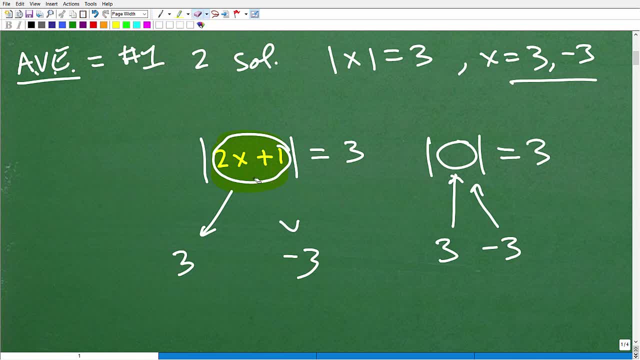 so, don't you know? you got to be, like, you know, uh, thinking big picture here, right. so when we are like, okay, how do we apply this, though? right. so we're like, okay, 2x plus one. i know you're either a three or negative three undercover, so i'm going to figure out what x is. so, all right, 2x plus one. i. 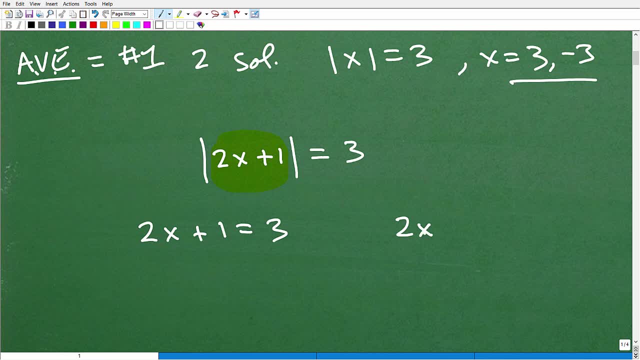 know you're either equal to three or 2x plus one. you're either equal to a negative three. okay, so this is how now we set up to solve absolute value equations: you take what's on the inside of this absolute value function and you set it equal to. 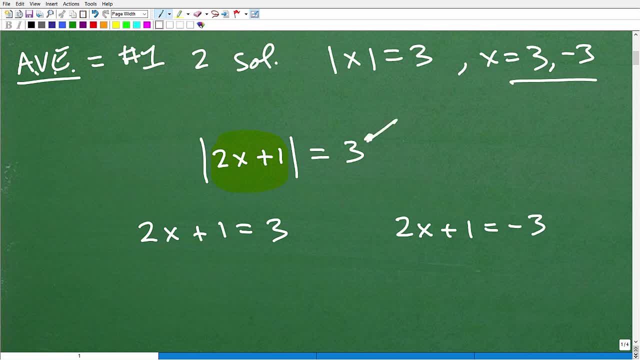 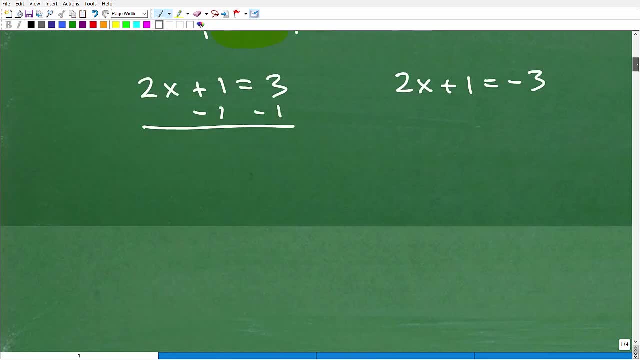 this one number. right, that's what we're doing here. all right, so now we just go ahead and just solve for x. i'm going to extract one from both sides of the equation and give myself some more room, and of course i'm assuming you're good with your equation solving. so we have: 2x is equal to. 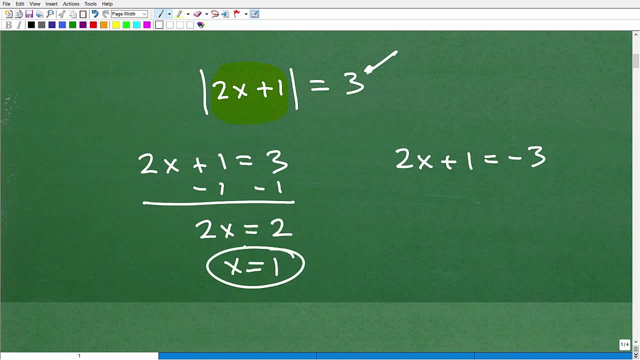 2 and x is equal to 1, so that's one solution. so now let's go ahead and continue this. we're going to subtract one from both sides, i get 2x is equal to negative 4. if i both sides equation by 2, i get x is equal to. 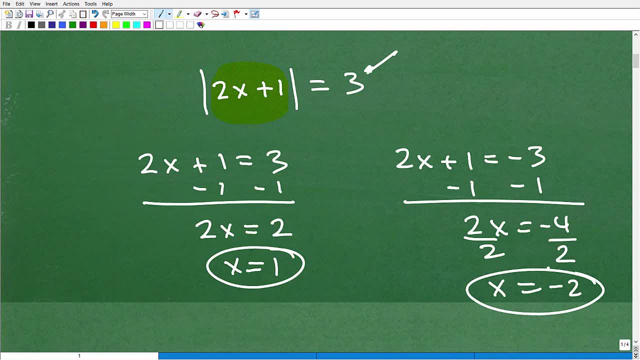 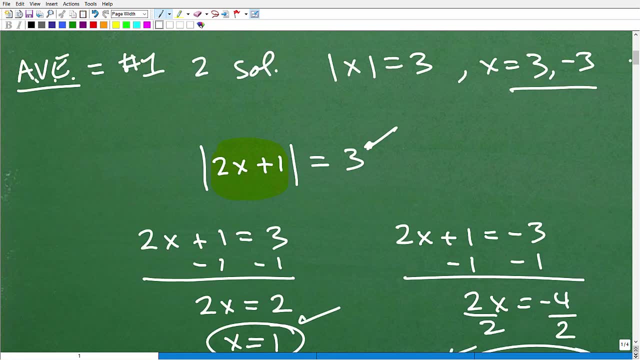 negative 2, and there is my second solution. so again, two solutions to an absolute value equation, right, all right. so that's what we're talking about right here. so that is the main, like the main concept. okay, you're gonna have two solutions and the way we're going to solve is we're going to set whatever is on the inside of that absolute 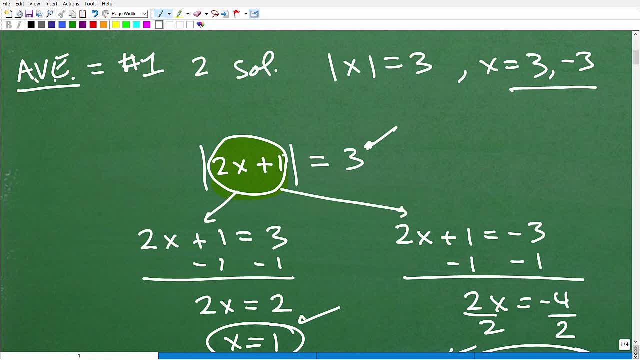 function. okay, we're going to take it out and we're going to set it equal to this value, okay, and then we're going to, uh, well, this value the positive and negative version of that value, okay, so again, you know, if you're just a little bit confusing, i would encourage you maybe to 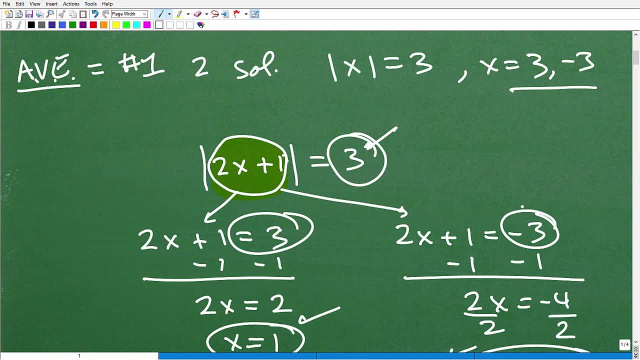 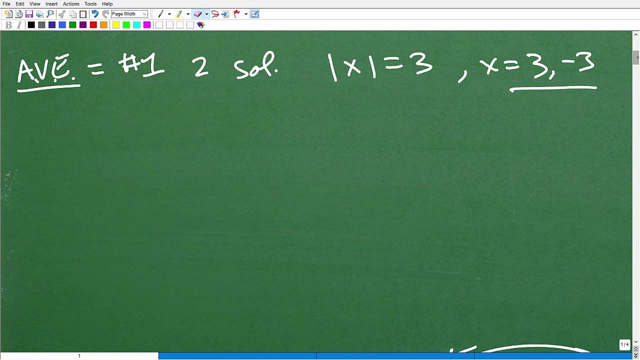 watch the video again. but uh, you know, once you, once this clicks and once the light bulb goes on, you'll be like: oh okay, now i got it all right. let's take a look at another example, because there is a few little twists here, not complicated, but uh, you know something that, some things that. 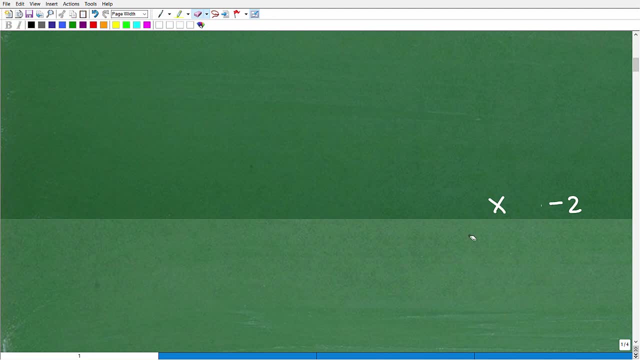 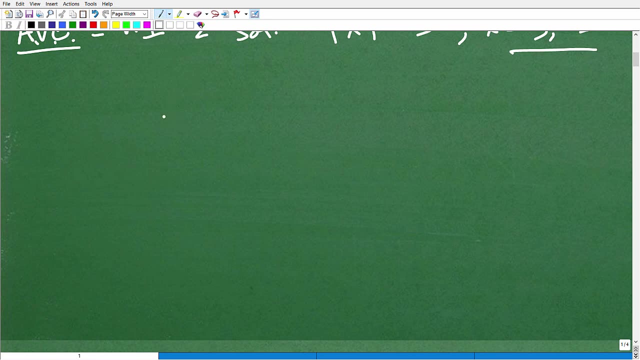 we want to let me erase this here. okay, so what about a problem? you're like, yeah, yeah, yeah, but what about these problems? well, you're probably thinking about something like this: what if i had two? absolute value of 4x minus 3? absolute value plus 1 equals? oh, i don't know. let's say um 11. okay, so what about an equation? 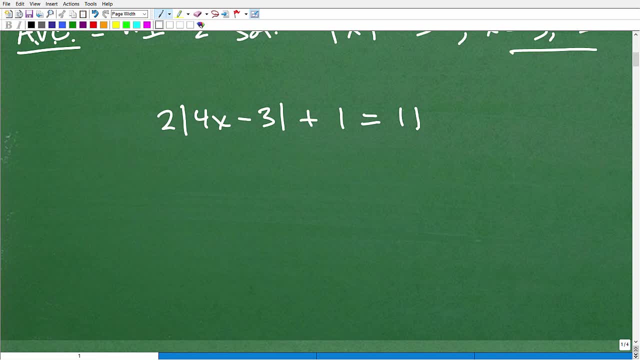 like this. all right, you're like: oh man, that's different, okay. well, here's the thing. when we set up to solve absolute value equations, what we want to do first is to isolate this absolute value function, get it all by itself on one side of the equation. okay, so we want to get this guy all by. 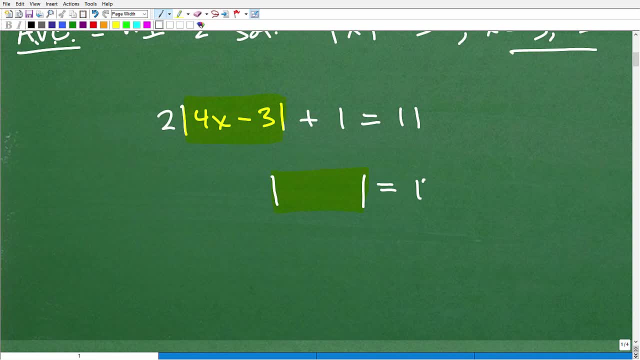 itself, no numbers in front of it, no numbers attached to it, and we want to get just one number. all right, once we do this, then we can set up, then we can take whatever's on the inside and set it equal to the positive version of that number and the negative version of that number. 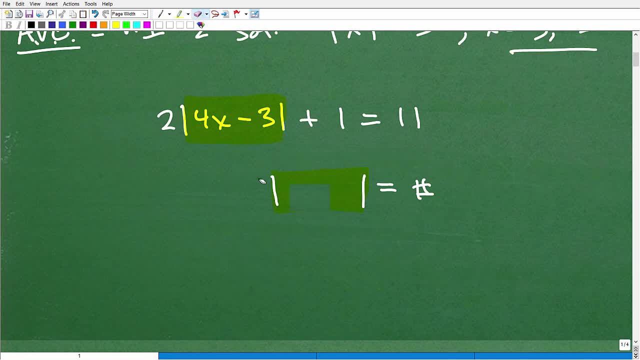 okay, so we're going to have to do a little setup work here, but it's no big deal. it's not the end of the world, so let's go ahead and isolate this now. when you think about that, this absolute value function, you're taking the same steps as if you were going to solve this equation to let's just. 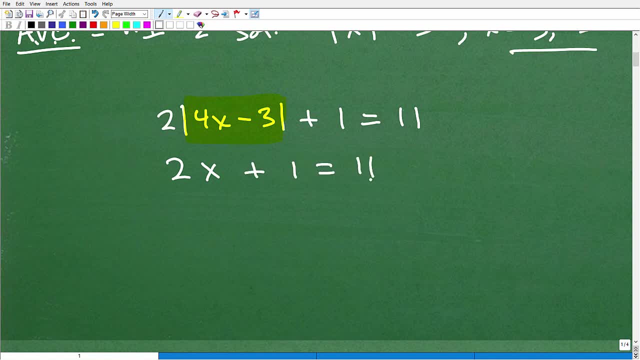 first take the x float addition and then pick up all the double chiefs and then you just divide that whole thing away. you just divide the whole equation by playing got big impossible. x equal between 12 and 2. expressed here, x once goes by: 11 plus 1 equals 11. how do i solve for x? well, easy i. 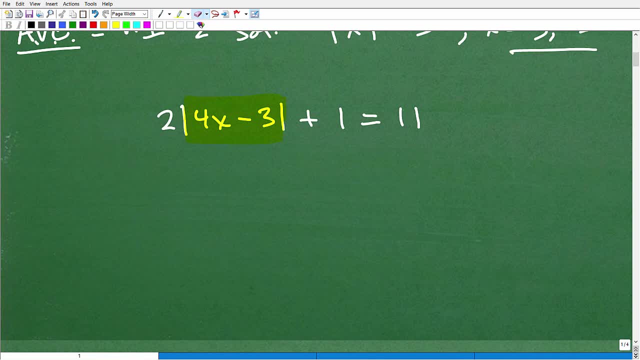 just subtract 1 from both sides equation and i have 2x is equal to 10. and then i divide both sides equation by 2, i get x is equal to 5. okay, 2 times absolute value of 4x minus 1 is equal to 10. all right, now I want to get: 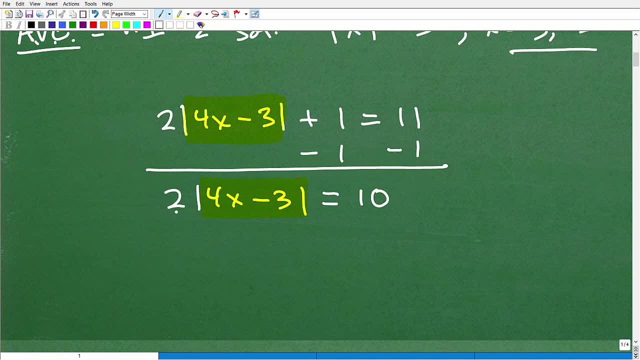 this all by itself, this absolute value function. I got this too, so I'm going to divide both sides of the equation by 2. all right now, another huge mistake students make. do not, do not, do not make this. this 2 only applies. in other words, when you're dividing, you can't do this. 2x minus 8. absolute value that, and 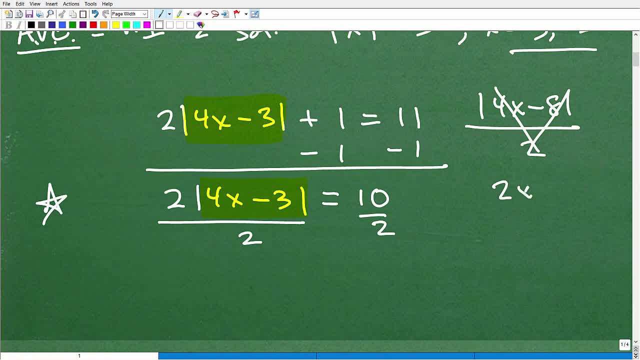 divide by 2 and you're like: oh, that goes on like this, and that is 2x minus 4. okay, wrong, wrong, wrong. okay that whatever is inside that absolute value function, leave it alone. okay, all this 2 is doing is dividing to this 2 here. so now I got. 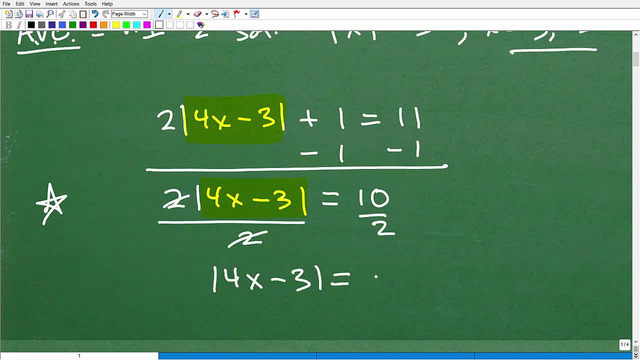 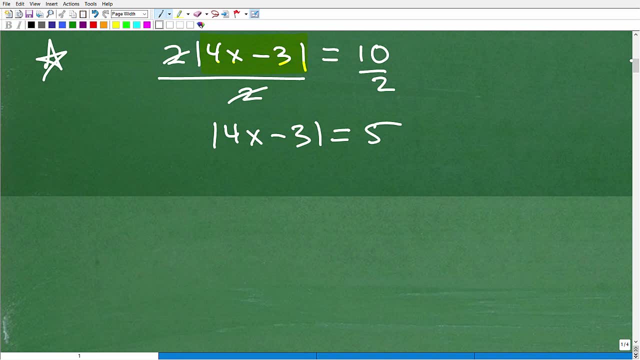 4x minus 3 is equal to 5. okay, if for those either are still with me, okay, you're gonna be glad that you you just didn't leave this video quickly, because I'm teaching you, I'm showing you the most common mistakes that students make when it comes to absolute values. 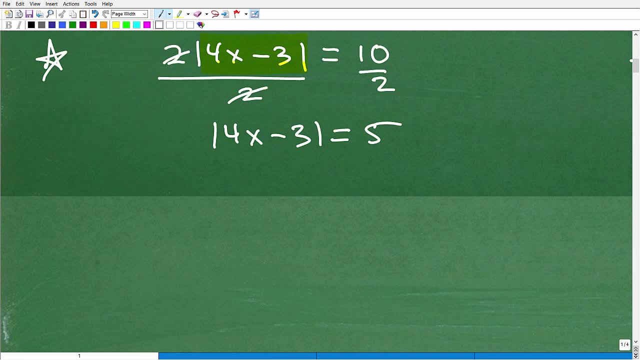 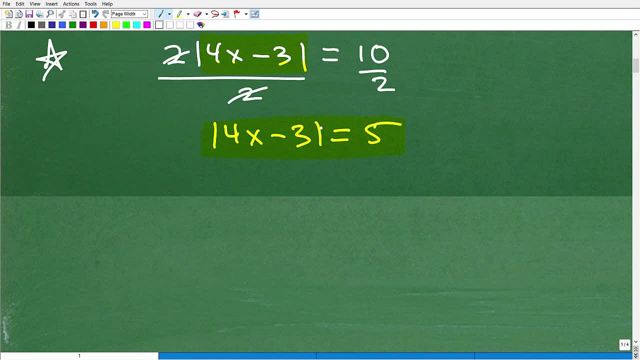 could set up to solve this. all right. so if there's nothing around this absolute value function, I got one number, so I'm going to take whatever is on the inside, which is 4x minus 3. I'm like, alright, 4x minus 3, okay. 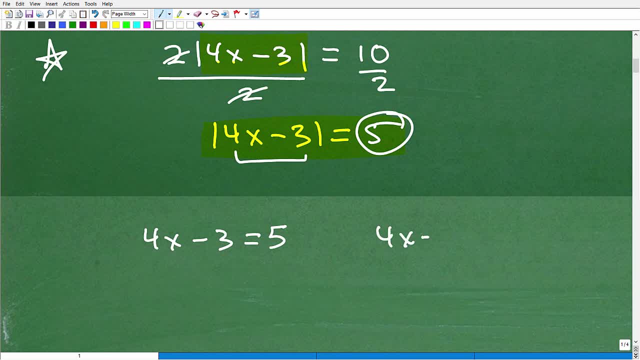 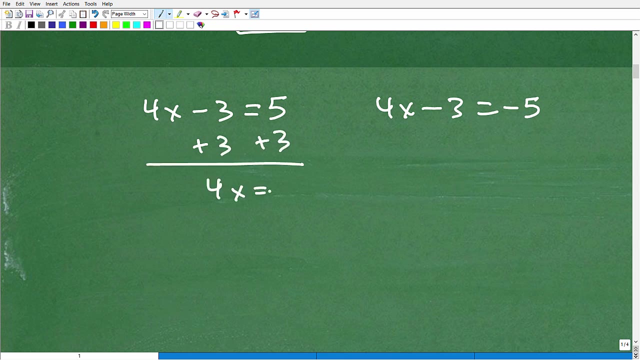 I know you're either a 5 or 4x minus 3 or a negative 5. okay, right, that look better. okay, so now we just got to solve for X. we'll add 3 to both sides here. then we got 4x is equal to 8 and X is equal to. 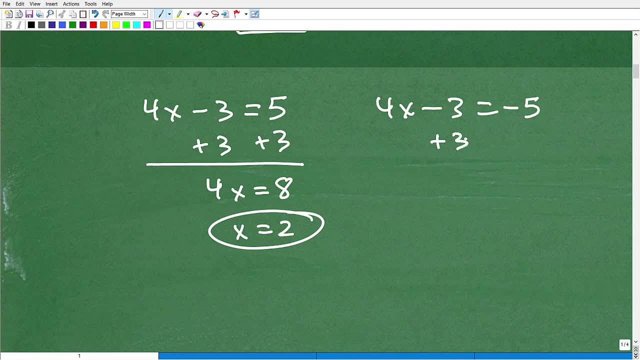 2. there's one solution and I'll let's add 3 to both sides of the equation. here I got 4x is equal- to be careful, right- the positive negative values here negative 2. so X is going to be equal to negative 2 over 4 or negative 1 half. so 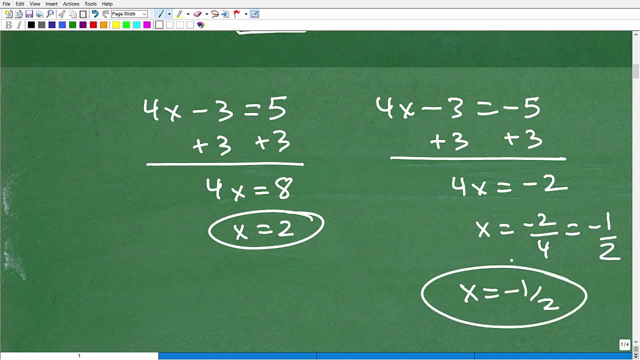 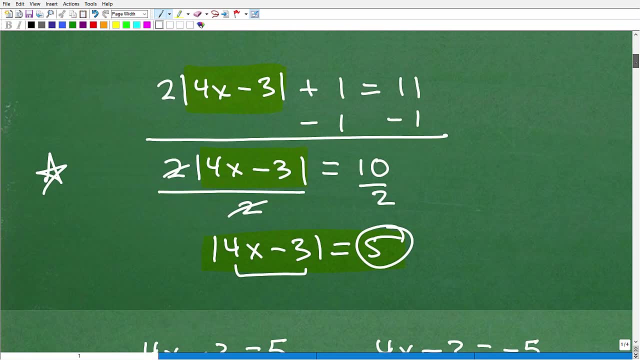 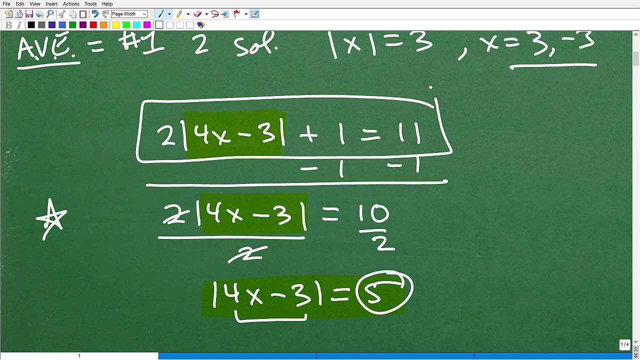 X is equal to negative 1 half. and those- and that is my second solution, and these here are my two solutions to this absolute value equation. this one right here. okay, all right. so absolute value equations very, very important. in mathematics, the concept of absolute value is extremely. 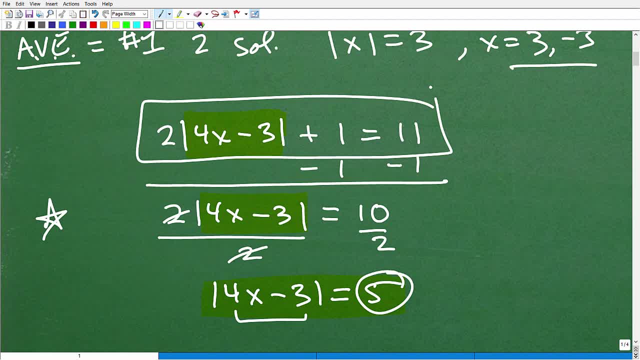 important and it doesn't go away. you're going to see, you'd like, when you're studying this stuff at this level, algebra, whatever class you're in, you're like, yeah, I've just got to get through absolute value. then I'll, you know, pass this test, pass this quiz. and then I'll just, you know, put that, put that behind.